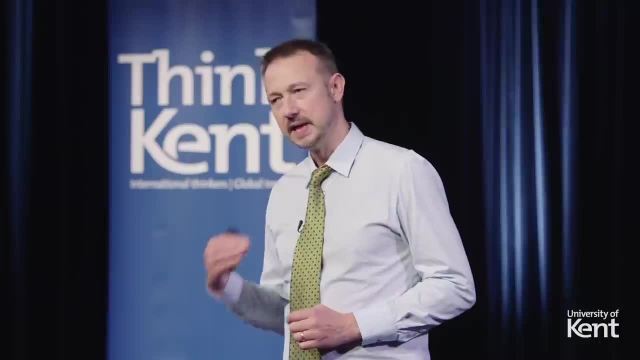 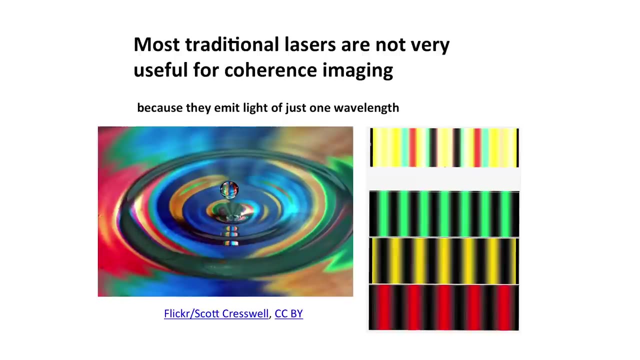 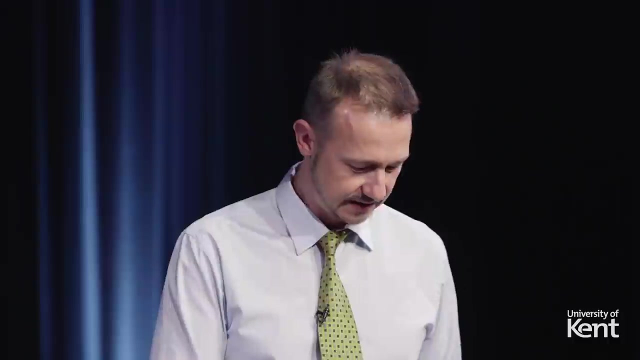 also be used to map different layers of tissue in the human body. So I want to talk to you about some of that. Now, the interesting thing about lasers, which are ubiquitous nowadays: we're constantly surrounded by them, and this is one such example of a laser. Those lasers tend to emit light at single wavelengths, single colours, And that is something to do with the way they're built. It's much easier to make a laser that does that, But we don't have much use for these types of lasers in the low coherence regime that. 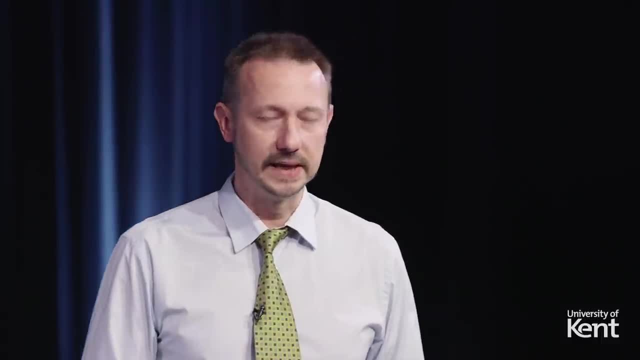 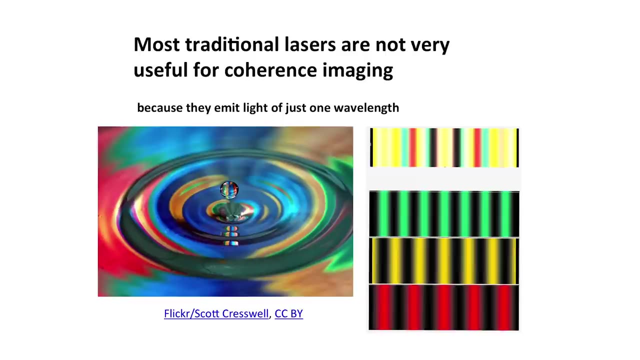 we use them in photography And let me explain why. If you look at the diagram on the right, it represents, if you will, ripples or interference fringes, which are created at different colours, And you can see that the spacing between them is really quite different depending on the 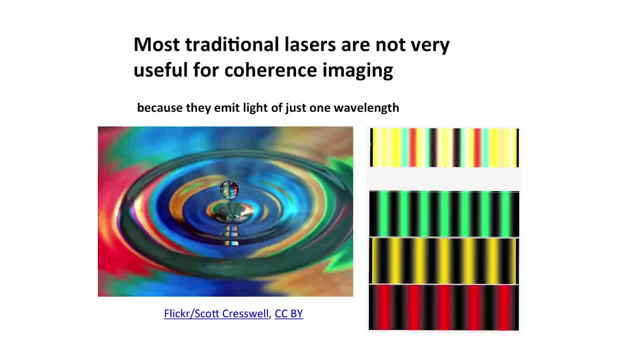 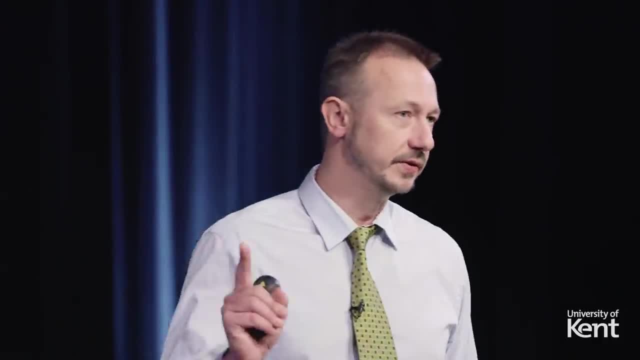 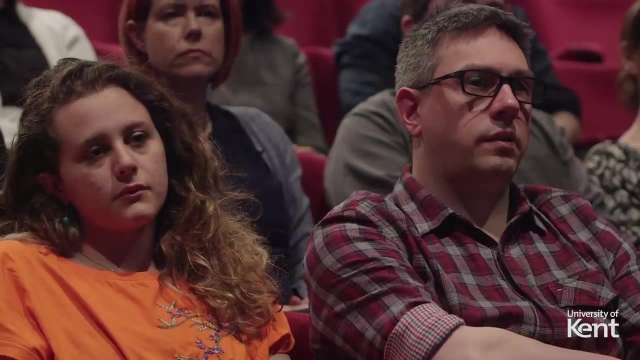 colour, And that's because the spacing between them is related to the wavelength. Now, if you want to pick out a standout feature in any of those lasers, you can do that by looking at the two of the black representations, the red, the yellow and the green. 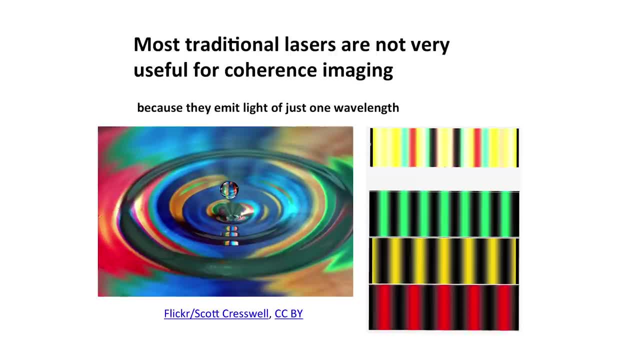 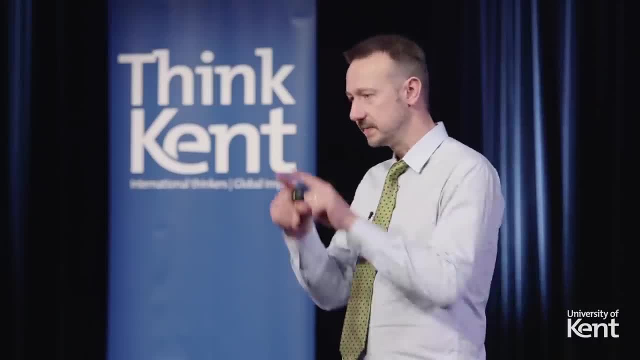 You will struggle to do so. However, if you overlap them. what they all have in common is that they have a central maximum in the middle of the pattern, And so when you overlap them, you will continue to have a central maximum, and then the ripples. 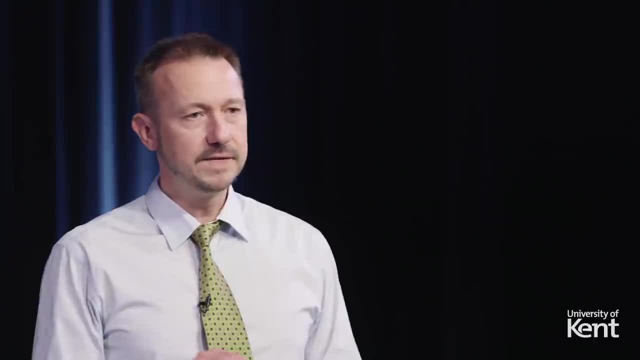 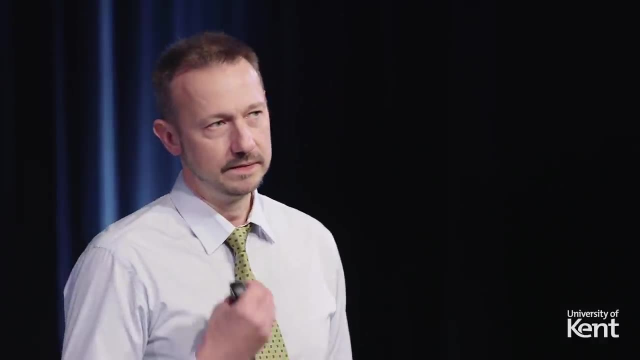 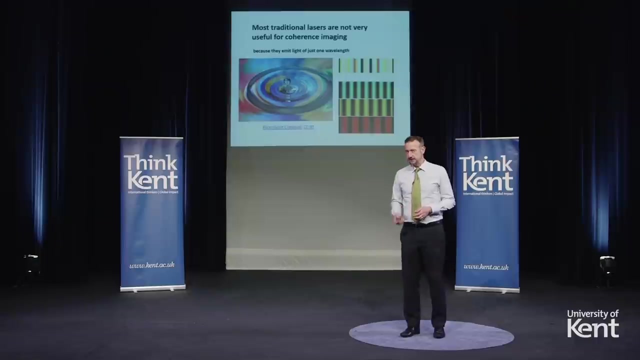 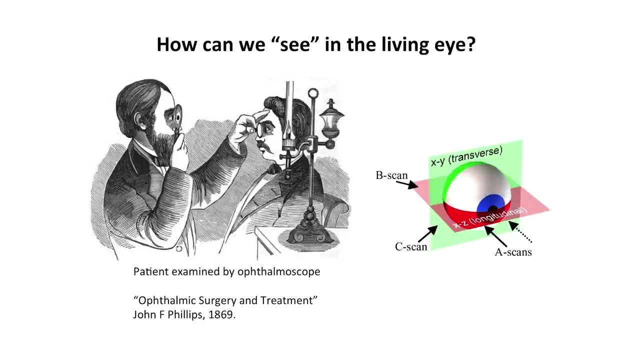 will go away and amount to nothing. All those features will just wash out away from the central maximum property of light, of low coherence light that we're trying to exploit in our research. As we do that, we build instruments which allows us to see into somebody's eye, for 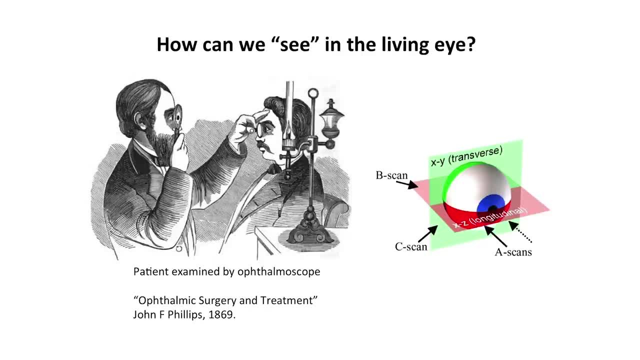 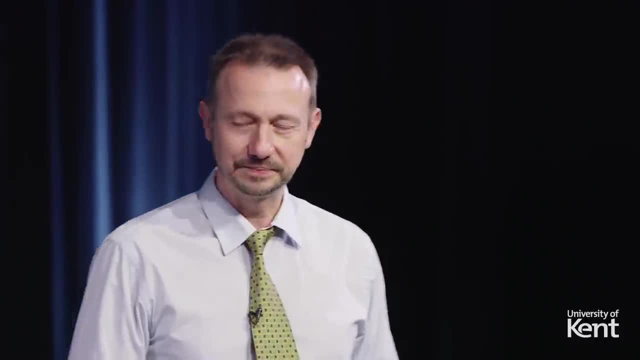 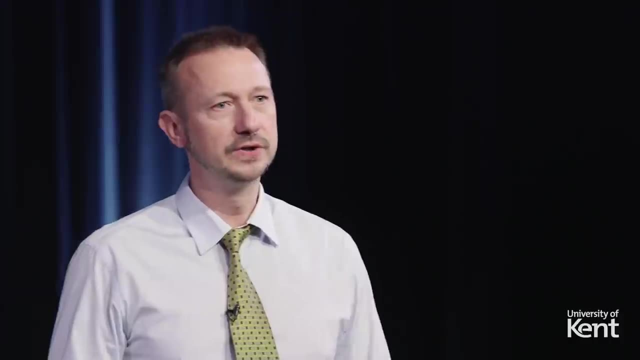 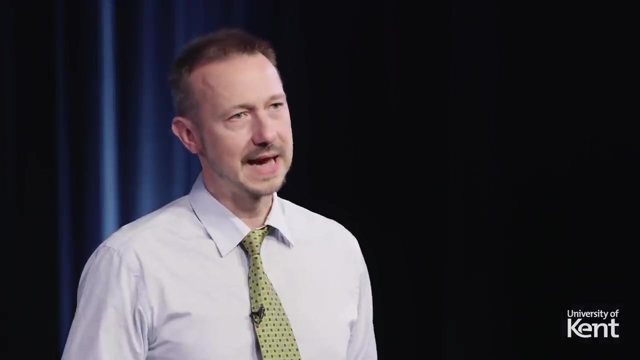 example, and our instruments look nothing like the instruments that used to be found in ophthalmology practices about 150 years ago. So when you examine features in a patient's eye nowadays, you'd be mostly interested in producing data in a number of orientations so that you give the ophthalmologist access. 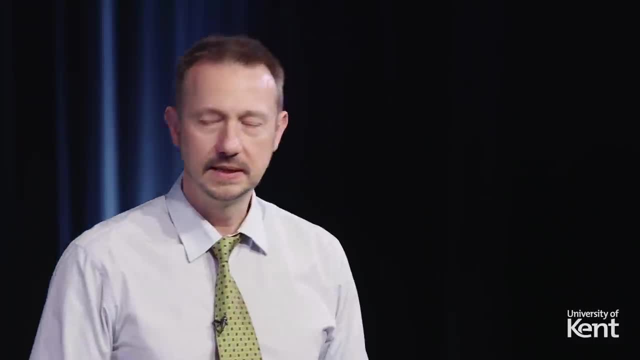 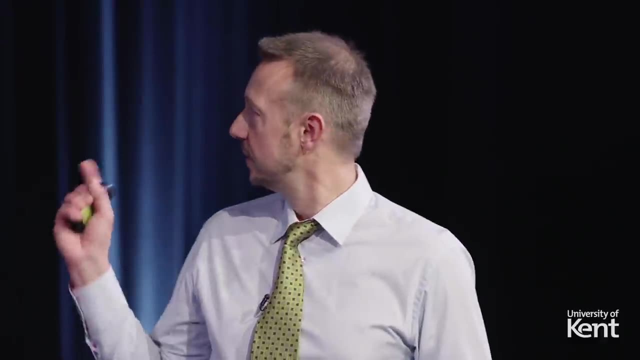 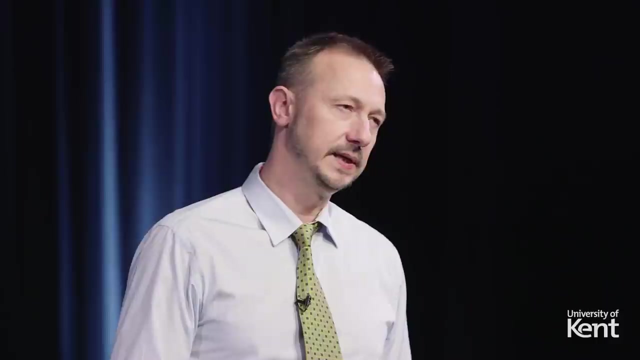 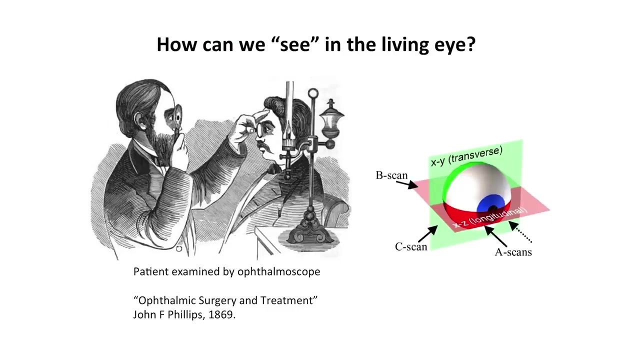 to a richness that allows them to then make an accurate diagnostic. And so I would point out to the three different orientations that correspond to much of the data that we display, And the clear distinction should be made between the horizontal, or what we call the B-scan. 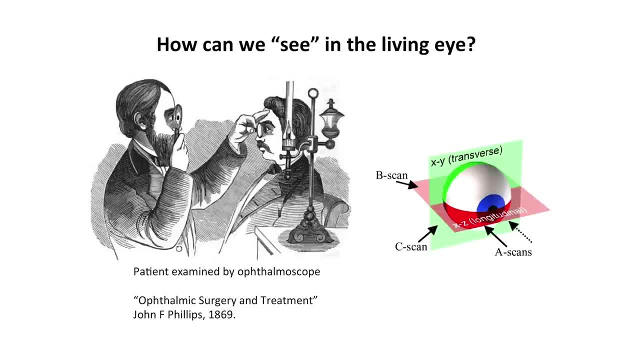 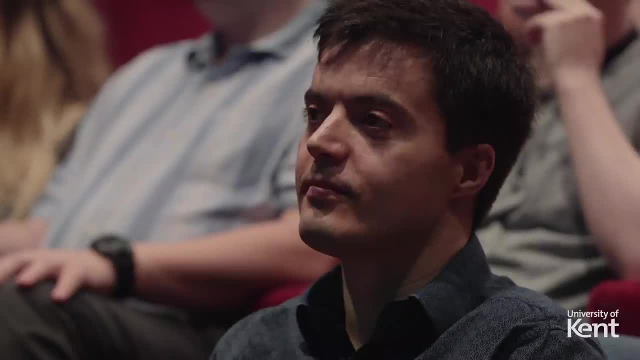 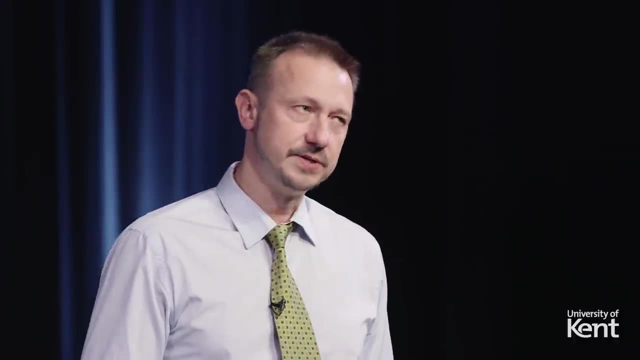 and the transverse, or what we call a C-scan. So that's the B-scan in pink there and the C-scan in green. And this is particularly useful for things like the eye, because there's definitely an advantage in being able. 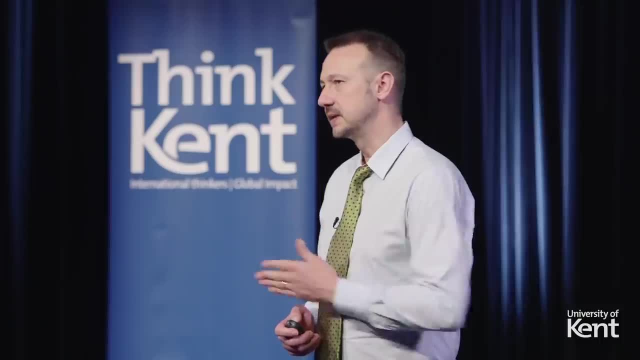 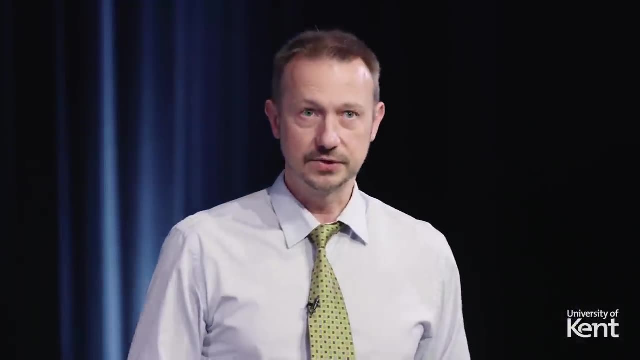 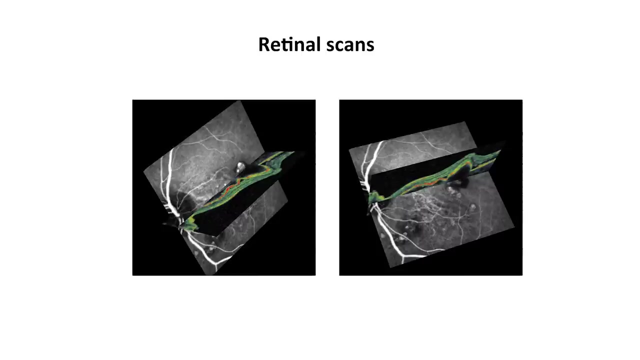 to show our types of images in the same orientation as those that ophthalmologists have learned about and trained to recognise. So much of my research has been devoted to finding ways to represent this information, this rich information, which is really three-dimensional information, to represent that in the different 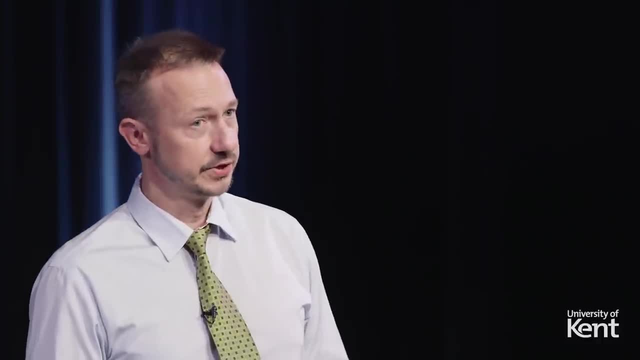 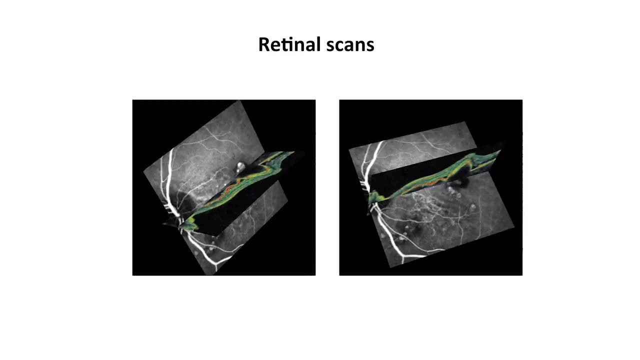 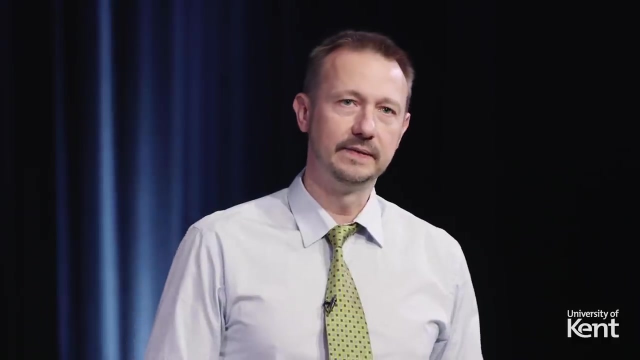 that would help the ophthalmologist make that diagnosis. As you can see, you could have the information from the eye fundus or the c-scan, shown in these diagrams in black and white or grayscale, and you can also have a b-scan depth information, which is often very illuminating. 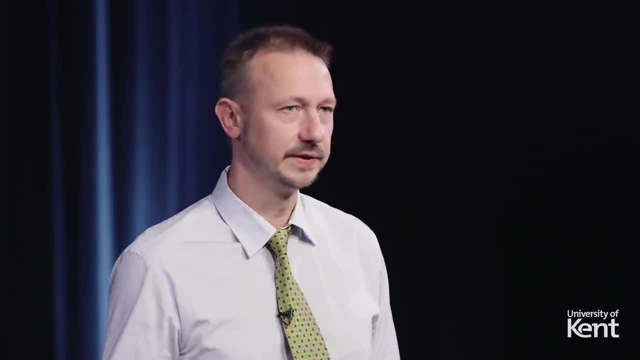 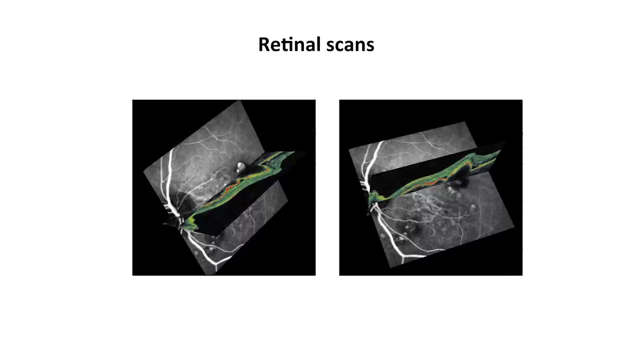 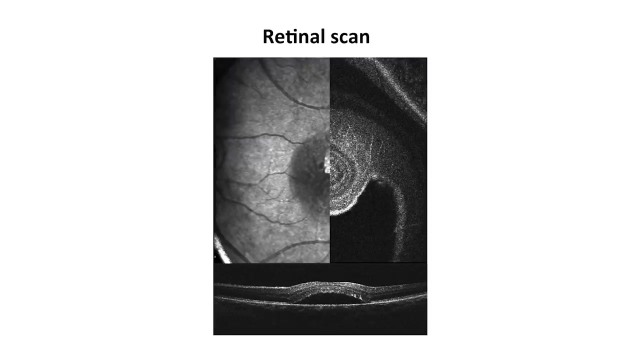 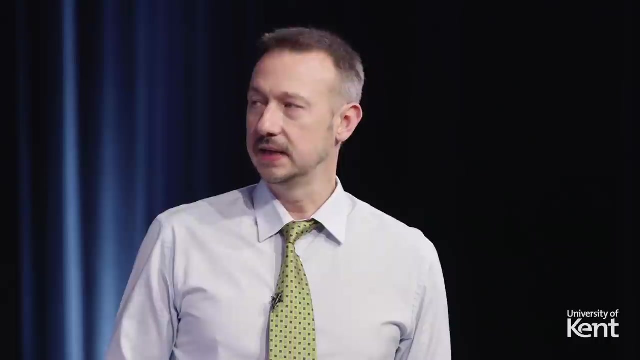 because it really gives you access to what happens below the superficial layers and that b-scan depth information is indicated by the color overlays. When you display that color overlay under the slice that represents the eye fundus, things become even clearer. so in this particular 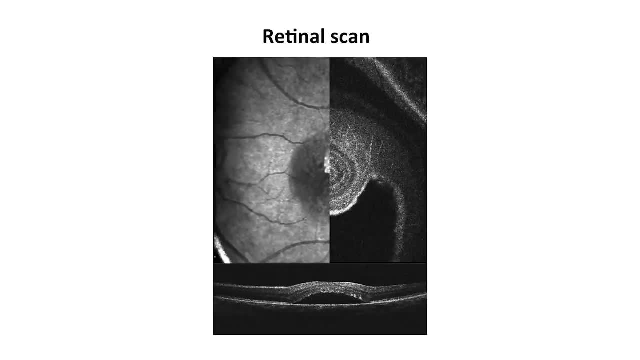 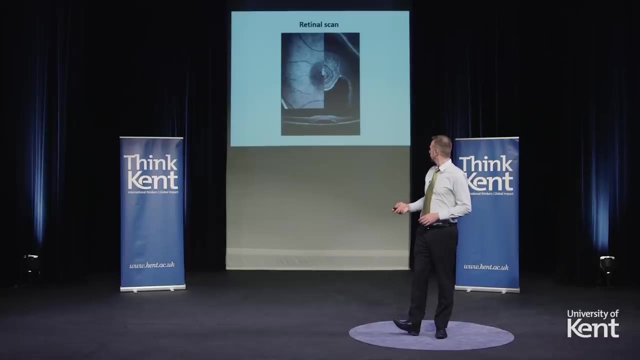 case we are able to see, for example, a retinal defect, where the retina layers are beginning to lift up and we see the eye fundus, And then we can see a little bit of a hole forming below the most superficial layers, And so being able to pick out features in either of these orientations is very important. 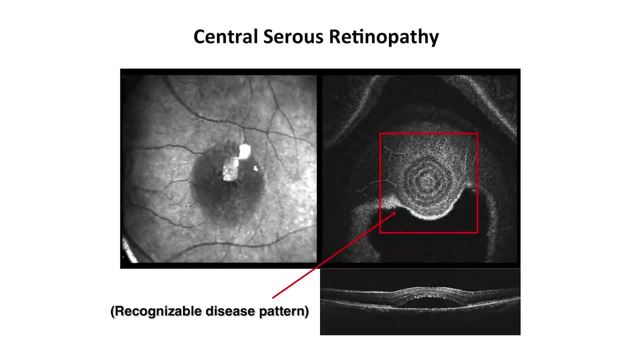 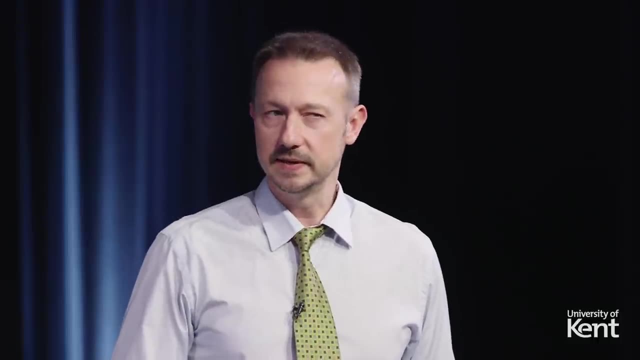 The ophthalmologist will often look for the pattern and in this particular case it's a disease, it's an eye condition called central serous retinopathy And we are able to see that recognizable bull's eye pattern, but only in the C-scan, only in the fundus image. 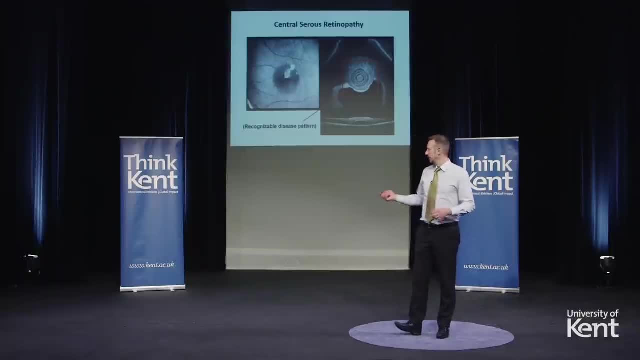 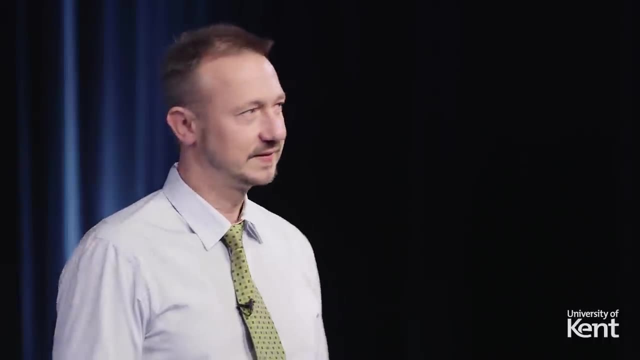 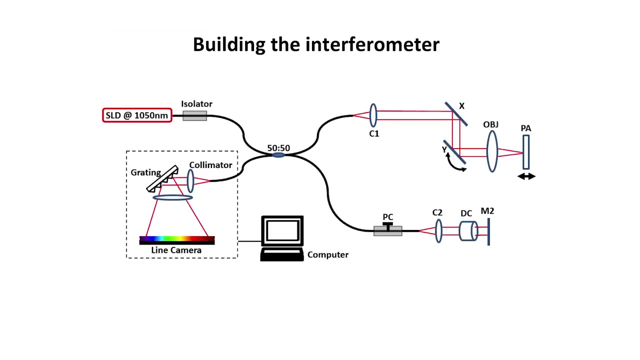 It's not so obvious when you look at the depth scan. So that's one outcome that we expect. but how do we ensure that we have the tools to produce such images? Well, we have to start by building an interferometer, And really the interferometer is just a very simple device. 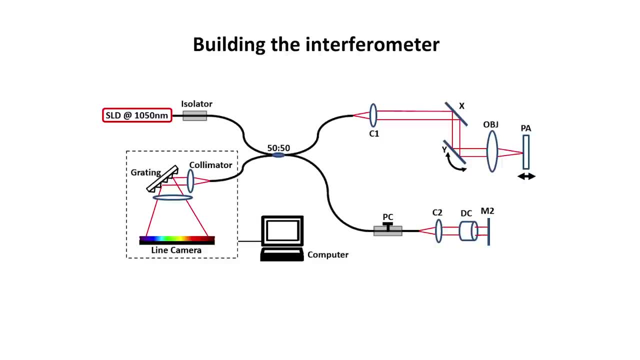 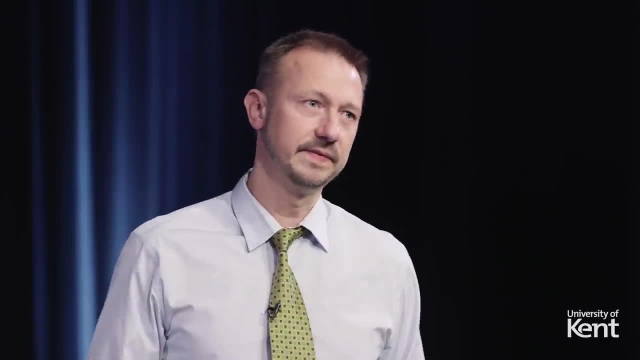 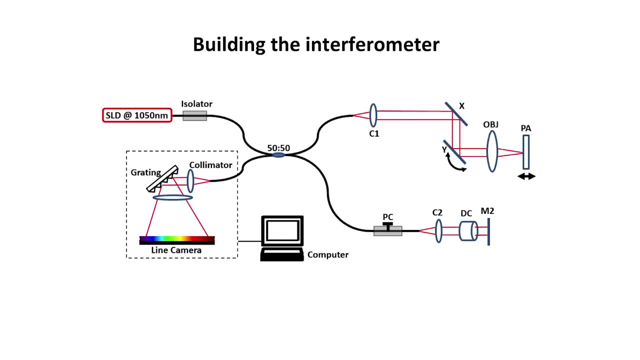 that splits light into two arms, an object arm or a sample arm, which takes light and shines it onto the feature of interest. In the previous case, that would have been the retina In the reference arm. meanwhile, light is propagating to typically a mirror and it returns. 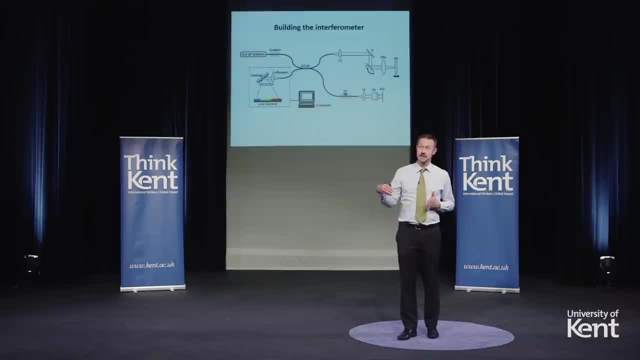 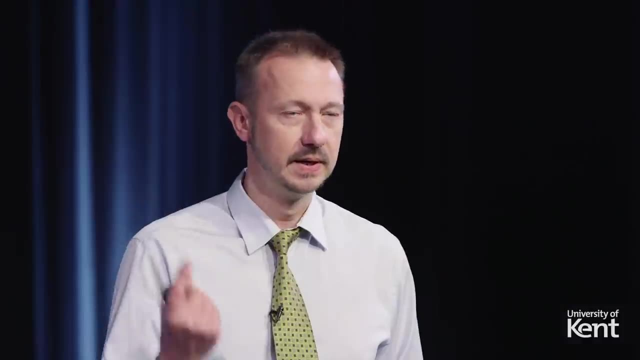 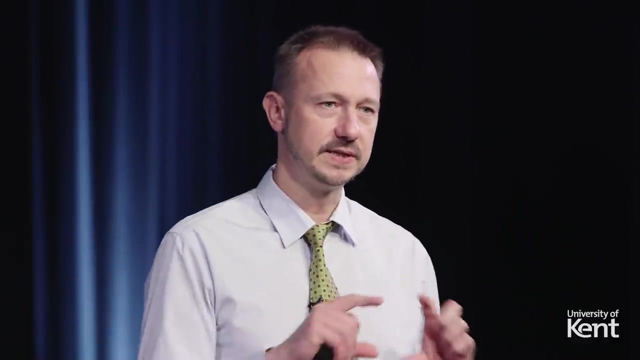 And then the two arms. light propagating in these two arms is allowed to interfere, And so the interference pattern will tell us. if you remember the previous slide where you saw the different fringes in different colours, it will tell us whether we're looking at a central maximum. 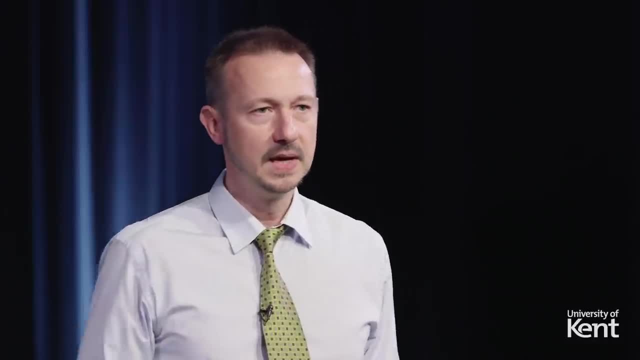 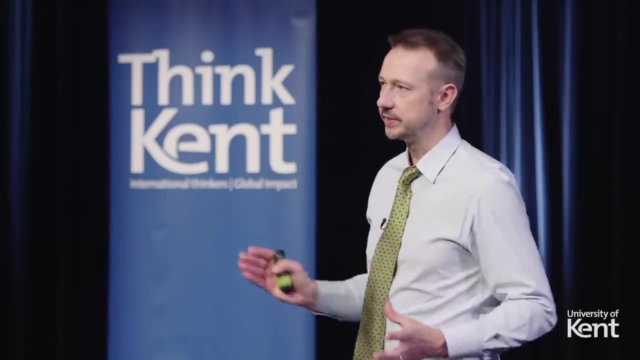 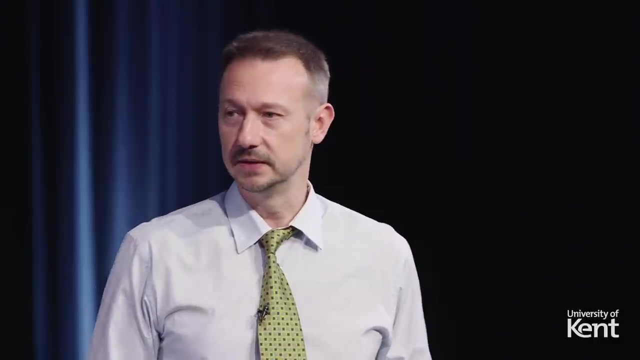 or we're out here in the wings and we're getting very little. So by doing that, at each location on the retina we can build an XYZ three-dimensional map of where things are essentially. Is there a reflection event happening at a particular location or not? 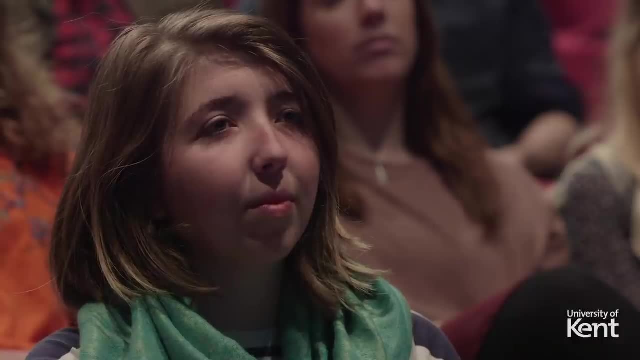 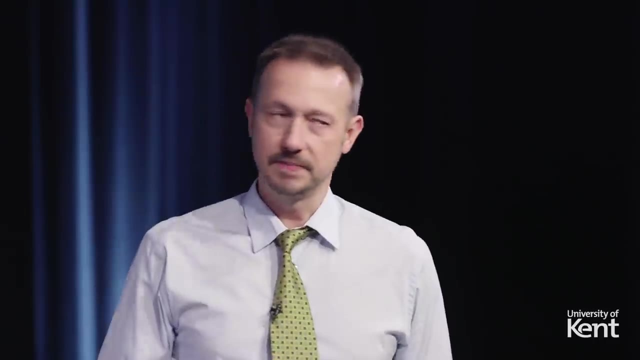 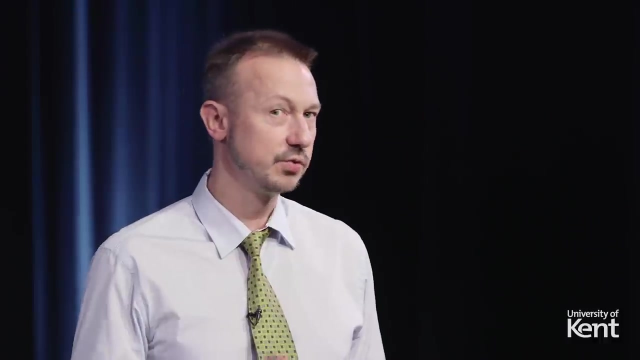 And if it is, how deep in the retina? Yeah, How deep in the tissue is it? And so we would typically detect the interference pattern with either a dispersive method, that typically spreads the spectrum onto a camera, or we could also have something called a swept source. 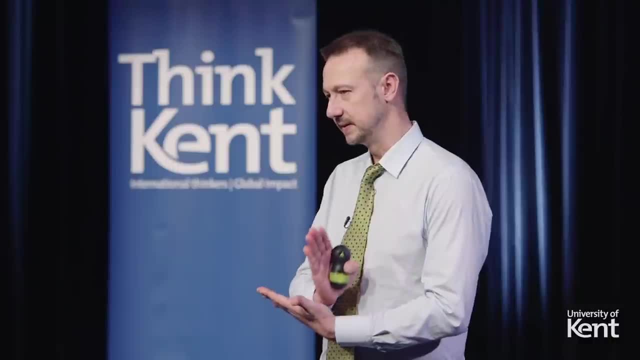 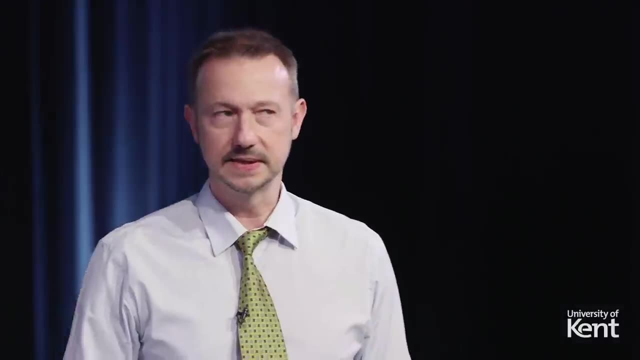 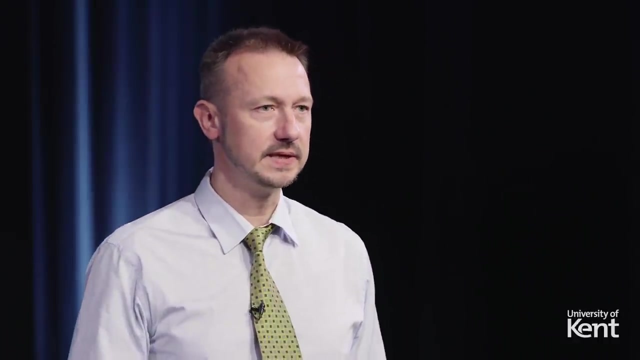 which is essentially a laser of a single wavelength that sweeps its wavelength very many times a second, typically a few hundred thousand times a second, or even faster than that. And in both cases we would be looking for these maxima of interference. And if we get that maximum of interference, 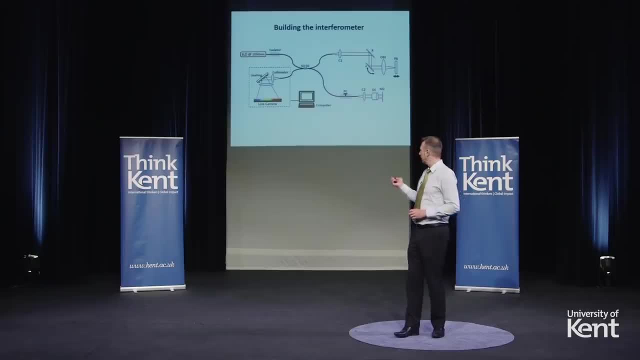 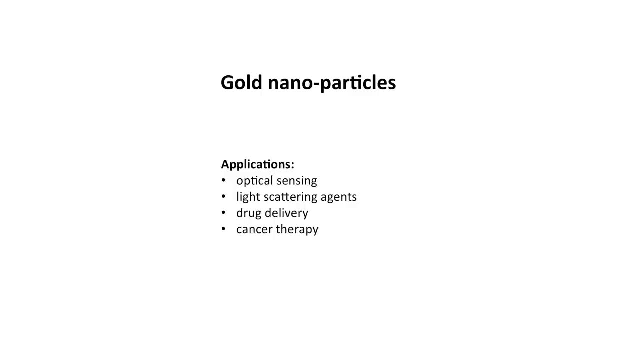 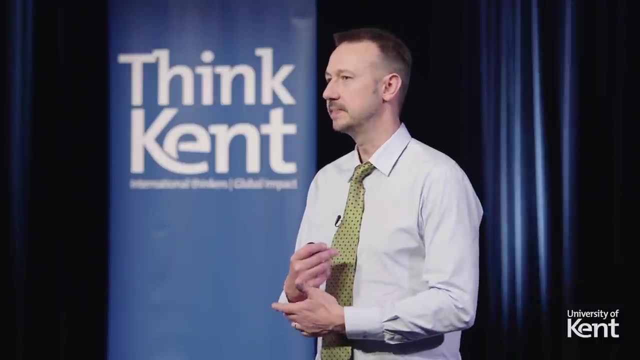 we can work out where things are And to extend our technique. we have recently started looking at reflection events from gold nanoparticles. Why do we say the extension of the technique? Because, in this particular case, we are able to produce um um. 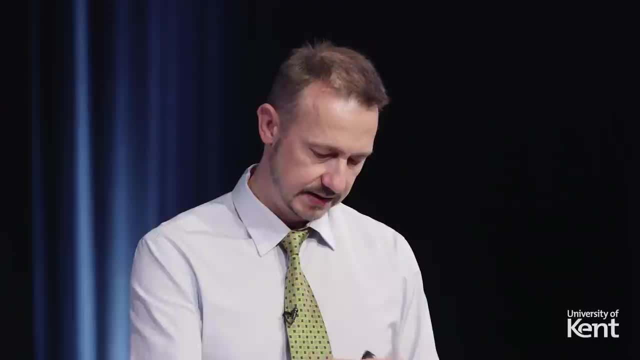 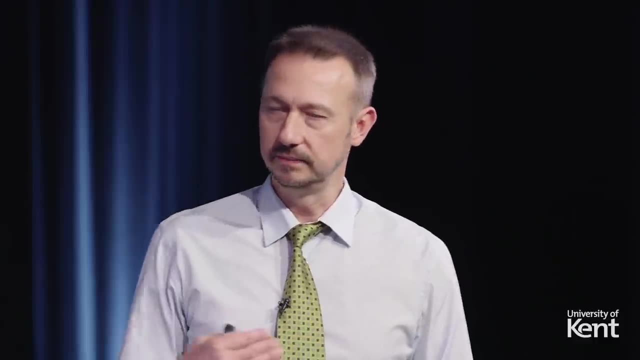 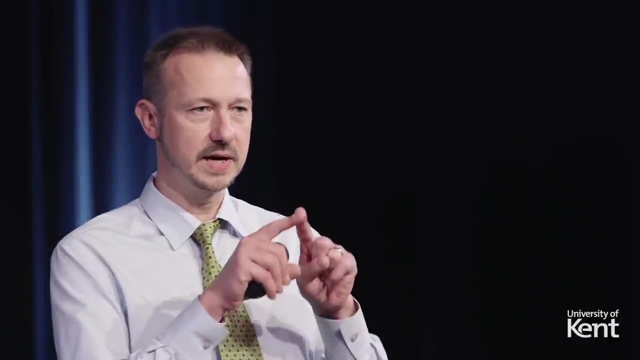 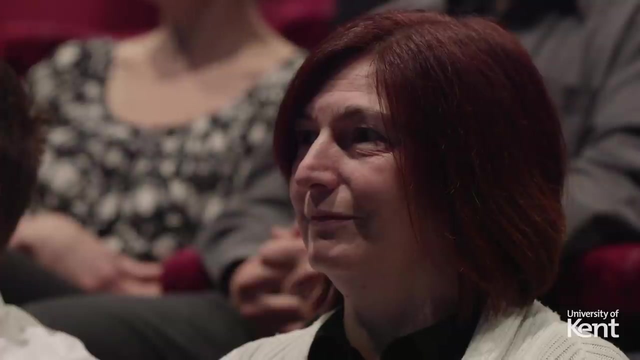 phase maps or information about the distance travelled, which is much more accurate than without the ability to measure phase. So measurement of phase is essentially measuring how wide one of those fringes is and where you are on one of the fringes. So we're getting down to very little. 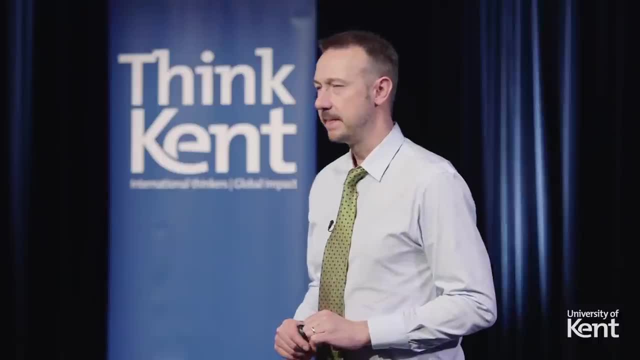 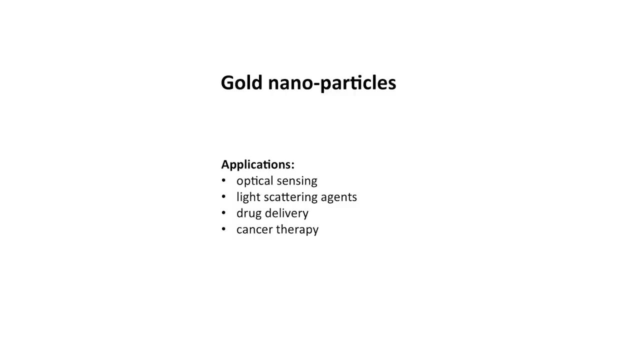 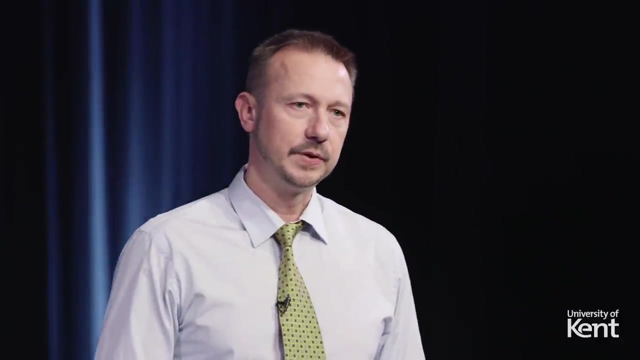 we're getting down to very fine displacement amounts. we're talking about nanometers rather than microns, So gold nanoparticles have this ability to migrate in the human body to regions where cancers are developing, and they have been used in therapy, because you can target the area with a near-infrared laser. 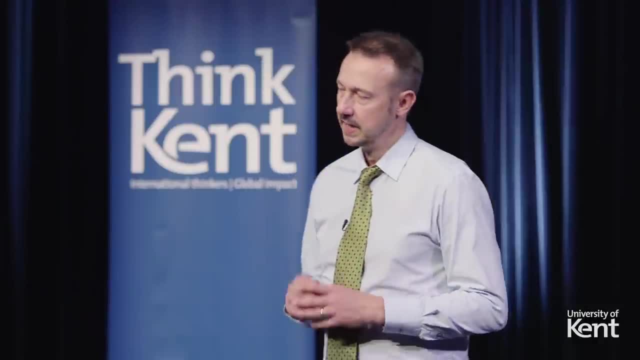 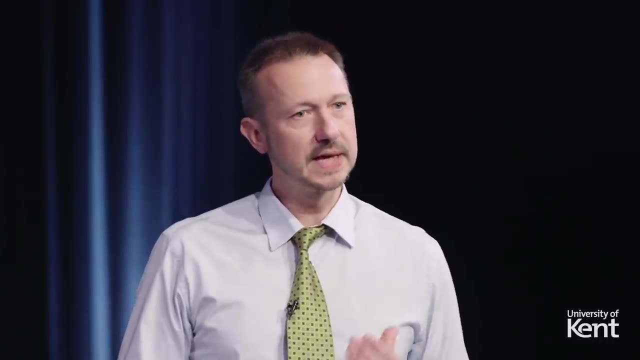 which causes them to heat up. they absorb very well in that region, causes them to heat up and to destroy cancer cells. But more importantly, we want to know exactly where they are and where is the highest aggregation of gold nanoparticles. So in order to do that, 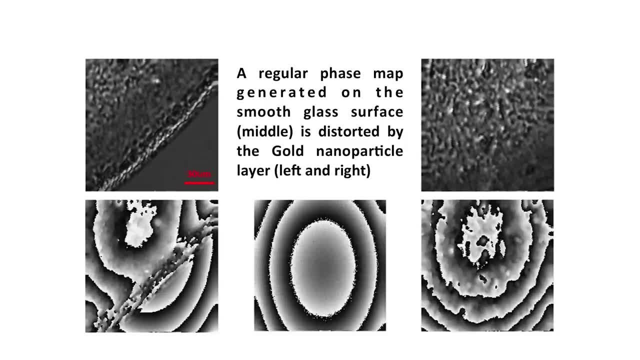 we have conducted a series of experiments where we placed these particles onto a slide and then illuminated them with a beam, just to see what sort of range of axial displacements we can expect If we just simply measure the thickness of the gold nanoparticle layer. 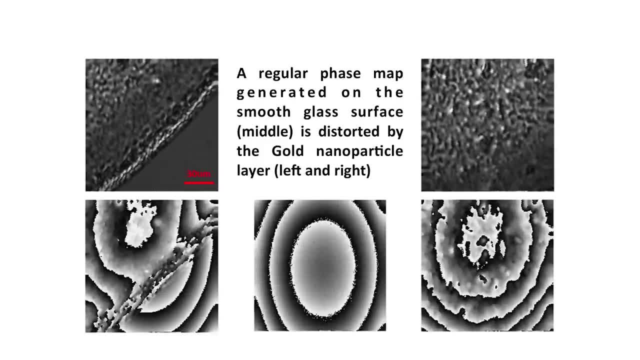 that is shown either on the left of the picture or on the right of the picture. we can definitely see some speckle in the image, some variation in the phase map, Whereas in the central picture we generally shouldn't expect, because that's taken from the smooth glass surface. 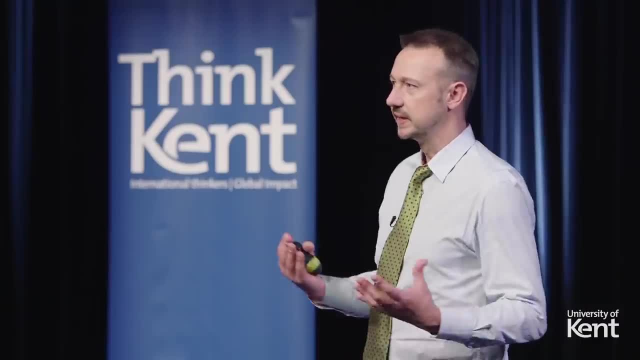 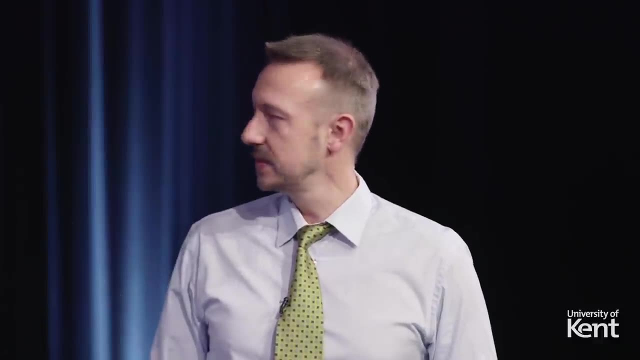 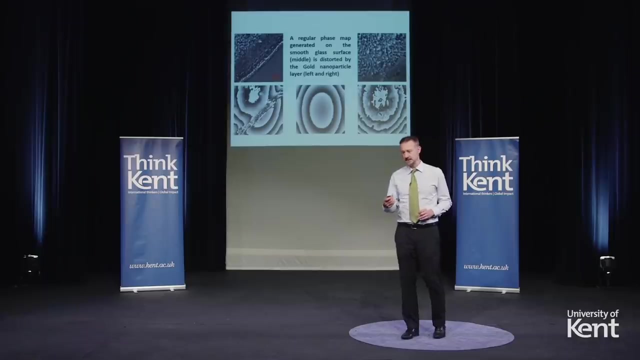 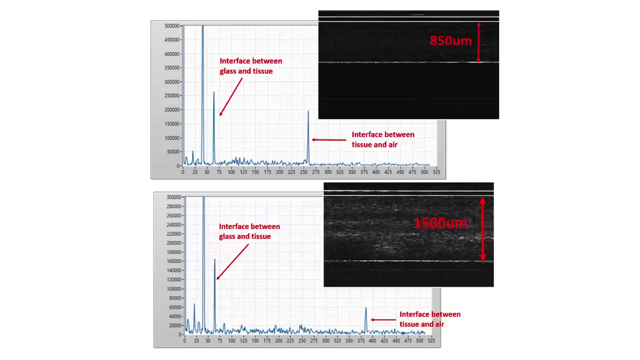 we shouldn't expect to see anything other than the bull's-eye typical fringe pattern that you might get as you scan. So having these phase maps gives us confidence that we can move towards detecting individual reflection events in depth, which we have done. And we can see that the top of the sandwich we created by placing a glass slide. 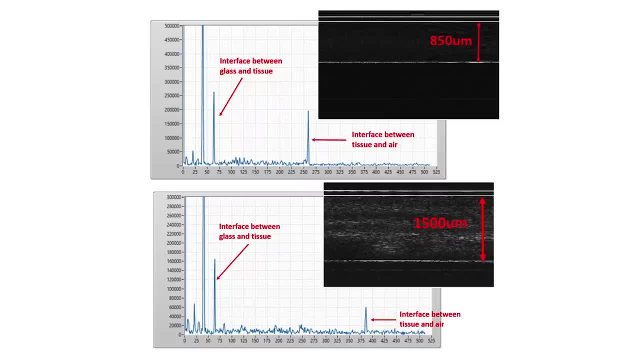 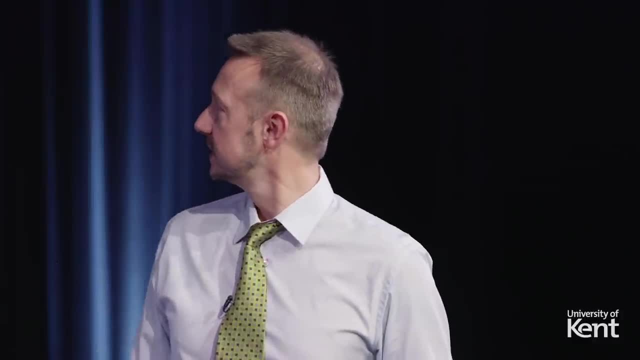 a microscope coverslip, in fact, on top of some real pork tissue, generates three different reflections and we can actually see the depth of all of these events. And we can actually see also just down to the nearest few microns or so. 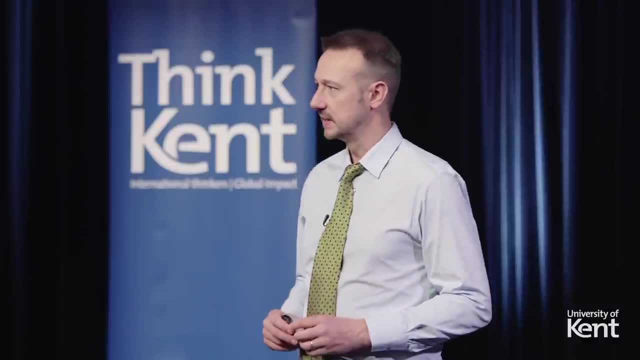 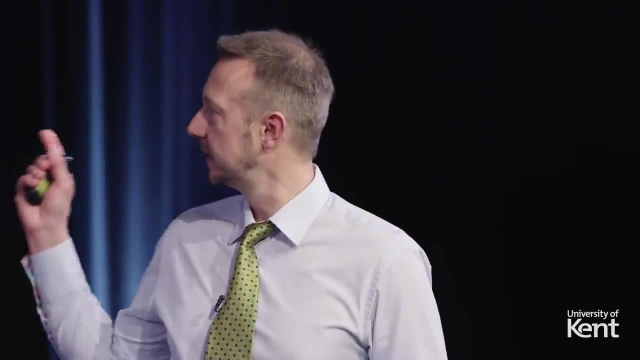 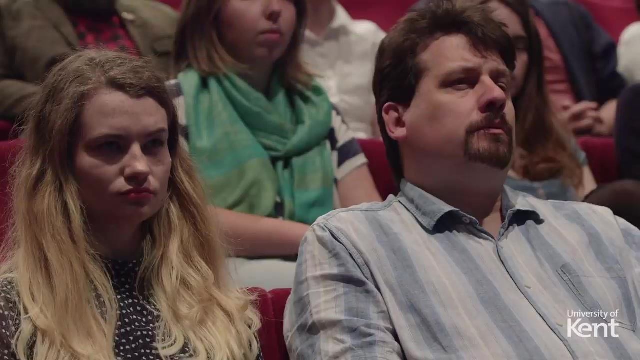 where the boundaries of the glass slide are, Where we hope to do. better is now to look at those boundaries and actually fix them to within a thousandth of the previous resolution. so just getting down from micrometres nanometre scale to nanometre scale. 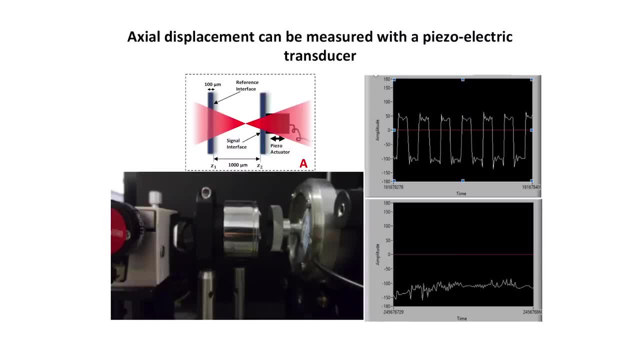 We can do that and we can calibrate our technique by using a piezo transducer, whose movement we control down to the nearest nanometre, and measuring the output in phase of that transducer, which is a graph we can see on the right of the picture there. 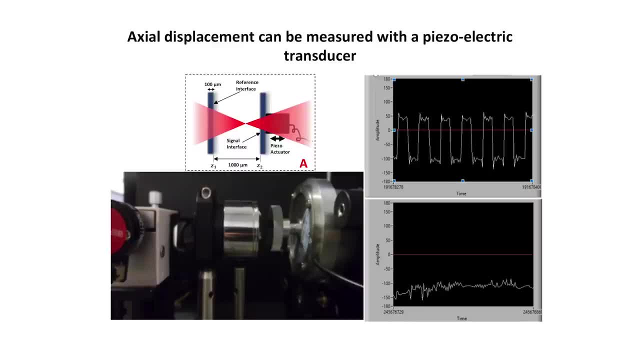 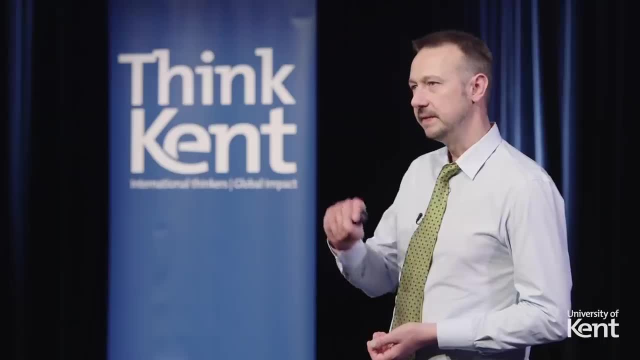 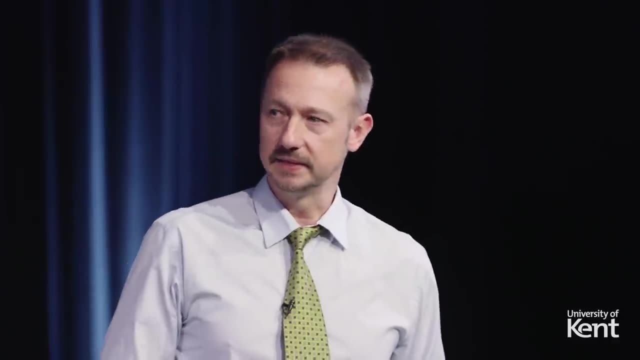 When we drive the transducer with decreasing voltages, we should expect that at the smallest driving voltage the phase output will be buried in noise, and that is our axial detection limit And, as I said earlier, that's typically a few nanometres. 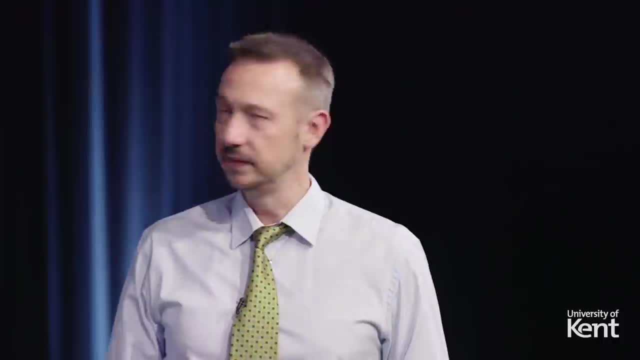 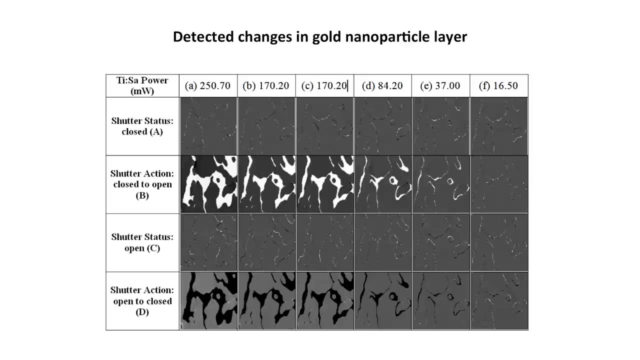 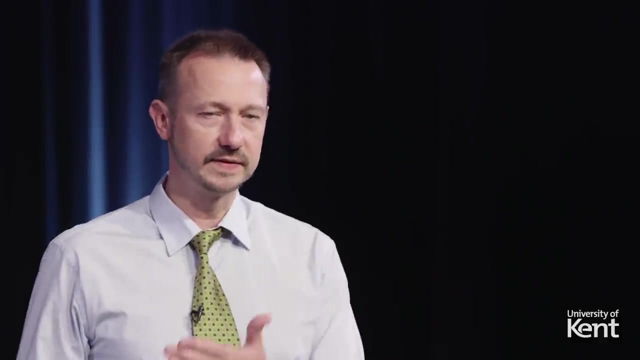 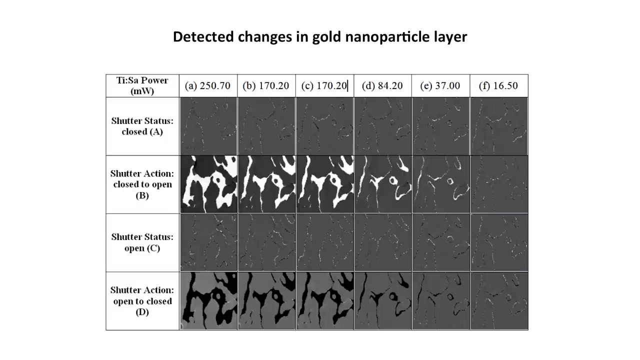 So we are able to see that with nanometre precision in the axial direction. So in our gold nanoparticle layer, as we produce the X and Y transverse, we're actually able to build pictures of the phase And we can see that the phase changes when the layer is illuminated.